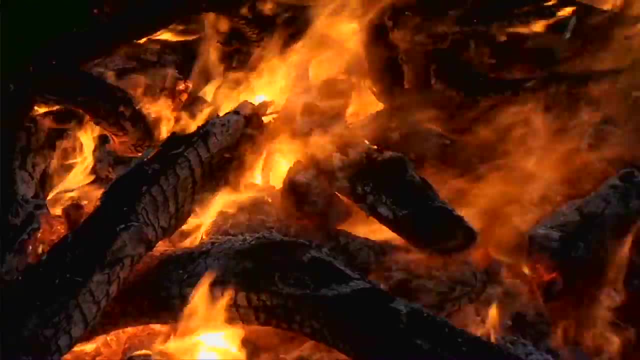 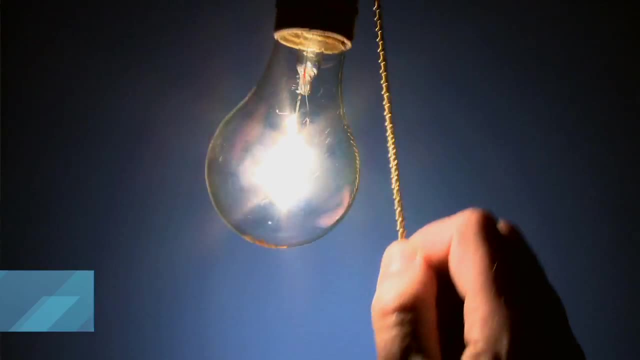 250 degrees C. When you stand by a campfire and see those glowing embers on the bottom, that temperature is about 1200 degrees C and the highest temperature that you would see at home is that filament in that light bulb is way above 2000 degrees C. 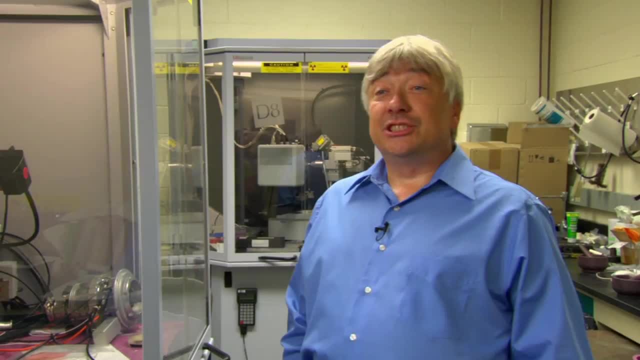 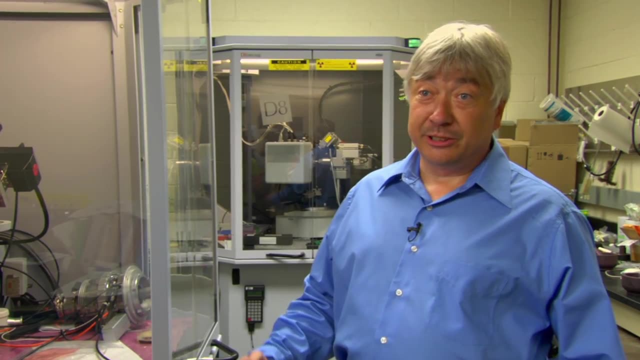 Another great property of ceramics is their hardness. Ceramics are very hard and, based on Mohs scale of hardness, the softest material is talc. the hardest material is diamond. The materials that we work with are very hard and the softest material is talc and the 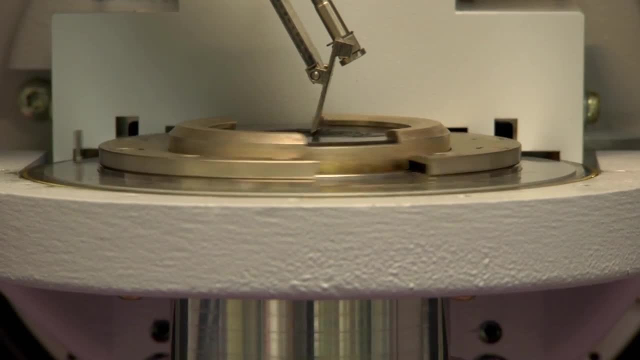 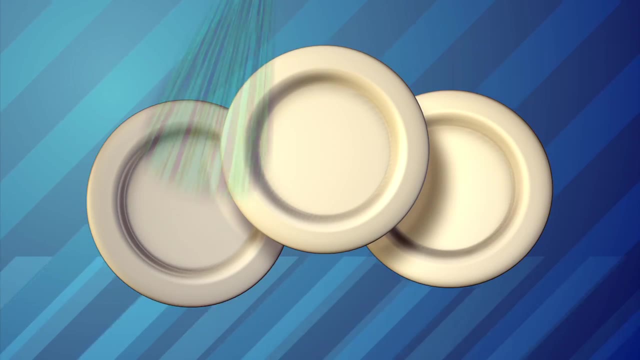 hardest material is diamond. The materials that we work with are very hard and the hardest material is diamond. If you need to cut something, you put ceramics on it and it can grind and cut almost anything. Ceramics can also withstand chemicals and erosion, But they're not perfect materials. 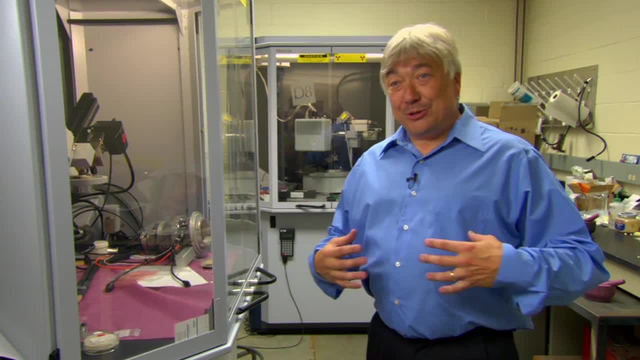 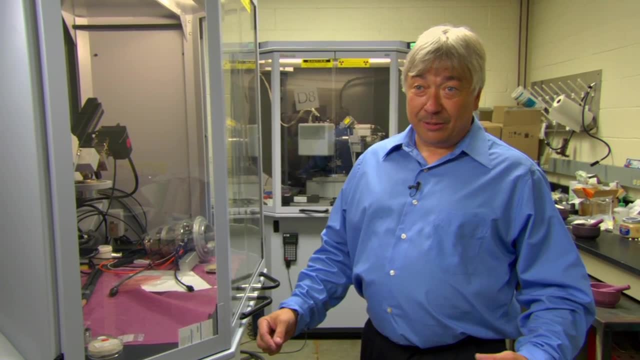 Unfortunately, they can be brittle and they can break. We try to make ceramics that try to get rid of the brittleness. That's the biggest drawback of ceramics. So we don't want to take something that we make, drop it on the floor and have. 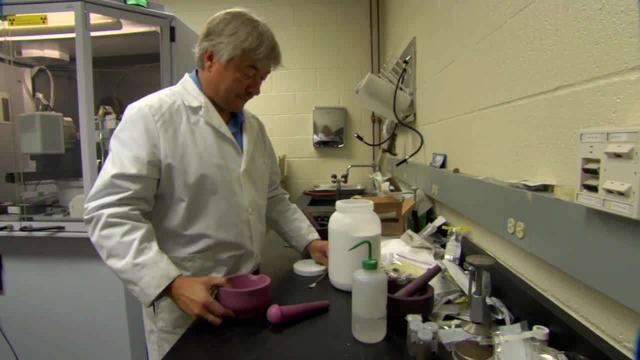 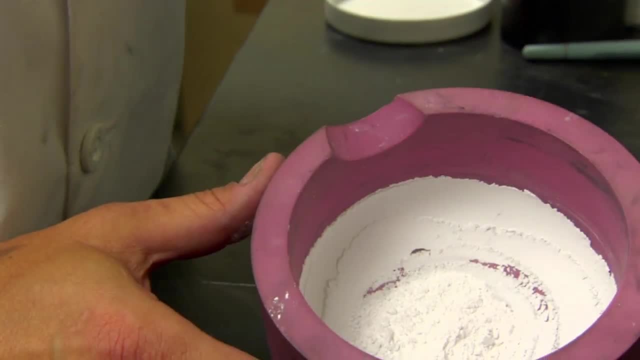 it break. Dr Zajkowski and his research team are working on a new type of ceramic. The team uses a process called sintering to create their ceramics. At our laboratory we use primarily dry powders. We mix two or more different chemicals, then 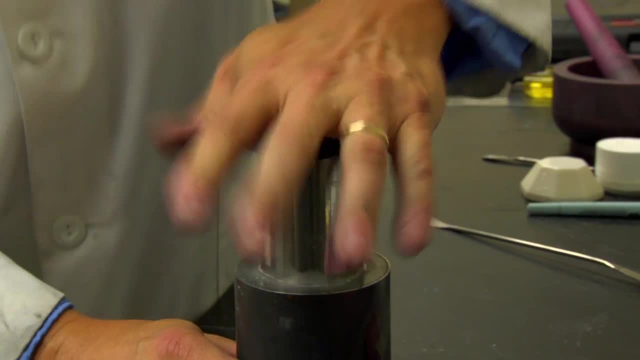 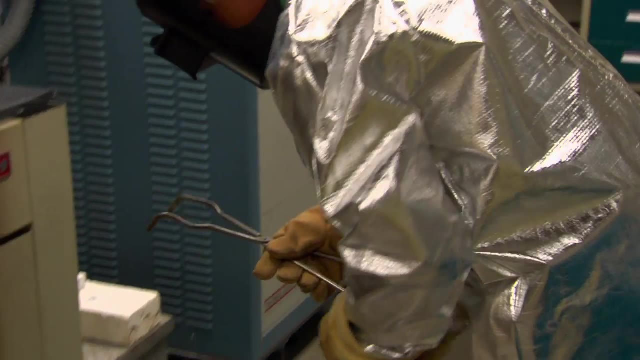 we put it into a mold and press it into a shape. It's usually in the shape of a disc, a thin disc. Then we take this disc and put it into a furnace. That's the most important part of making a ceramic is to put the material into a furnace and put tremendous heat on. it. You have to heat it between 1700 to 2200 degrees. That's the most important part of making a ceramic is to put the material into a furnace and put tremendous heat on it. You have to heat it between 1700 to 2200 degrees. 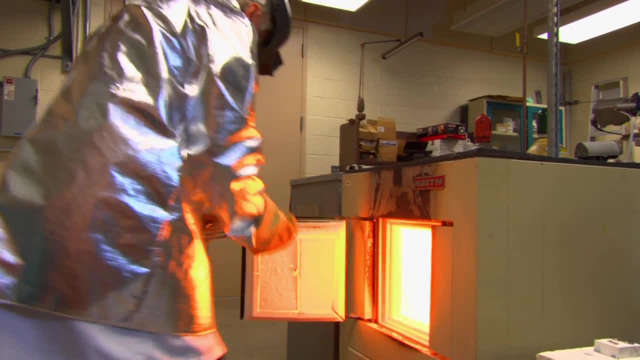 That's the most important part of making a ceramic- is to put the material into a furnace and put tremendous heat on it. You have to heat it between 1700 to 2200 degrees. They heat the disc to just below its melting point. That causes the powders to stick together. 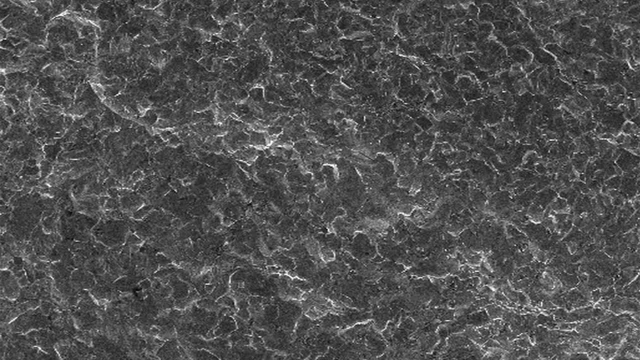 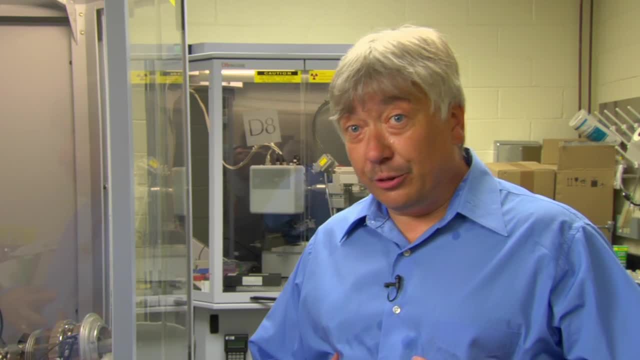 and form a strong crystal structure. Now it's a ceramic. Ceramics are going to be with us forever and they're going to be used in many, many applications. We are particularly looking at ceramics for Navy applications in engines. We want to put 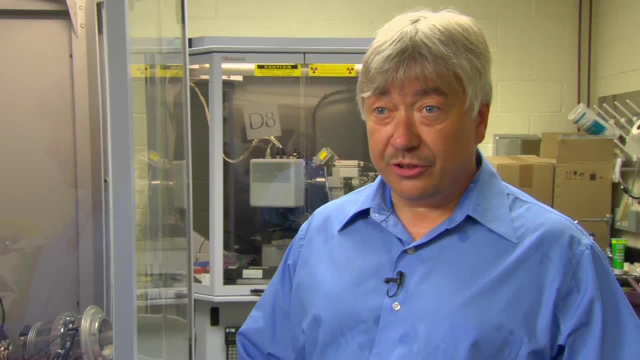 ceramic materials in there. that allows the engines to operate at higher temperatures and derive greater efficiency from the fuel. Dr Zajkowski and his team have received a lot of feedback from the team. Dr Zajkowski and his team have received a lot of feedback from the team.